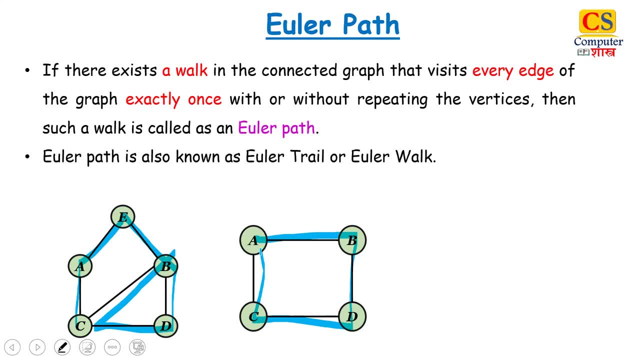 And we have covered all the edges at once. Again, this is an Euler path. There is one more example Now. in this example, if I start from E, Then I can cover one more edge. You can take any path, but you cannot cover more than two edges. 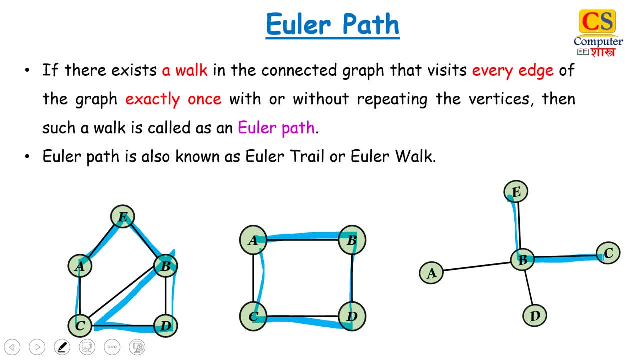 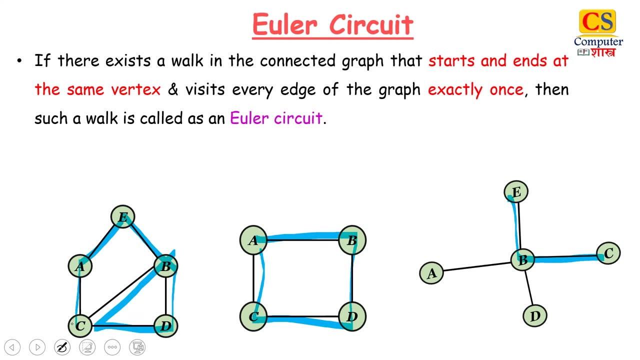 So this is not an Euler path. So this is the concept of Euler path. Next we will see what is Euler circuit. We will check the same examples Now, if there exists a walk in the connected graph that starts and ends at the same vertex. 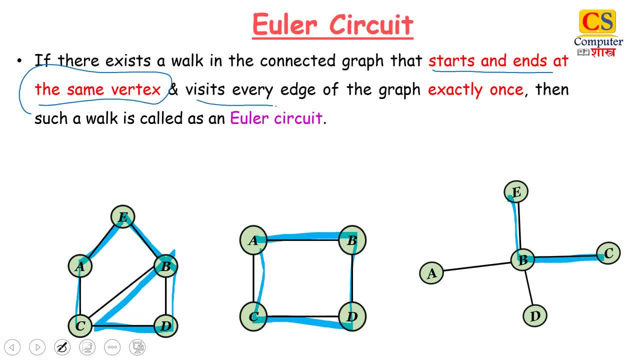 That means it should be closed And visit every edge of the graph exactly once. The properties of our Euler path should be that we have to visit all the edges exactly once. We can take vertices as many times as we want. The only condition is that it should end at the same vertex from where it started. 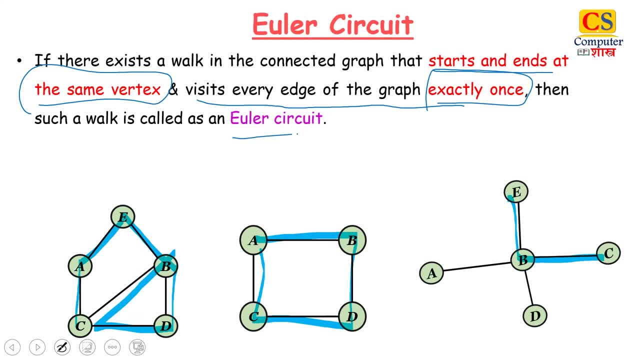 If there is such a walk in your graph, then it is known as Euler circuit. So can I say that a closed Euler path is called as an Euler circuit. Closed Euler path means it ends where it started. Now Euler circuit is also known as Euler cycle or Euler tour. 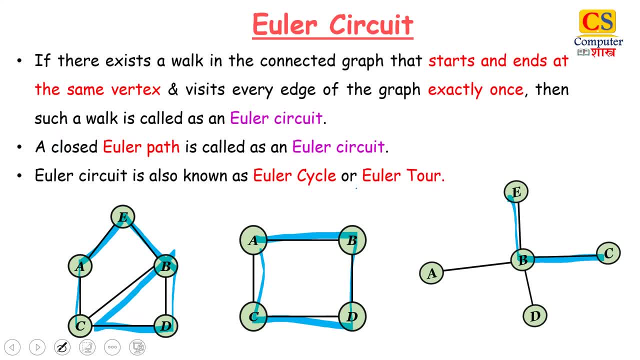 Now we will check in three graphs whether we have Euler circuit or not. Now, in first graph we started from C and ended at B. Both are not identical vertices, So first is not an Euler circuit. In second we started from A and ended at A. 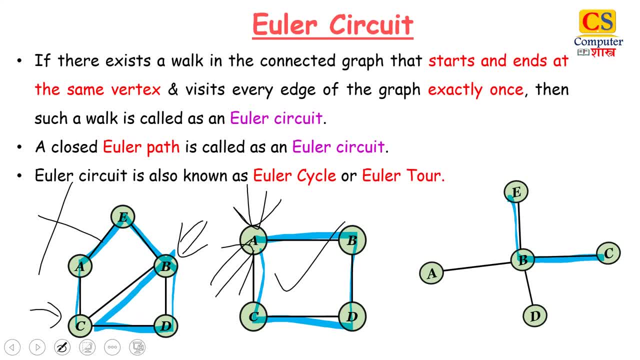 So this is Euler circuit. In last graph our first condition is not fulfilled, that we have to cover all the edges. So last one is also not an Euler circuit. So among these three graphs, only middle one is an Euler circuit. When we did Euler path then we saw that Euler path is in first and second graph and not in third. 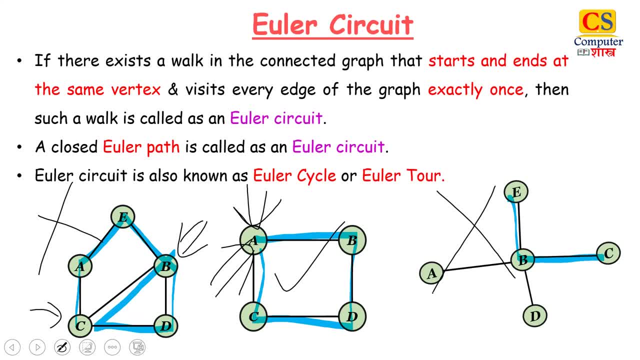 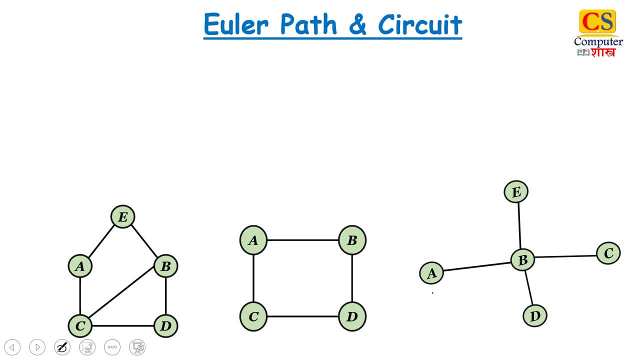 So I hope you understood the difference in path and circuit. Next, we have two theorems to check whether any graph is an Euler path or not. Is there an Euler circuit or not? Because this is a simple graph in which you can see whether an Euler path is made or not. 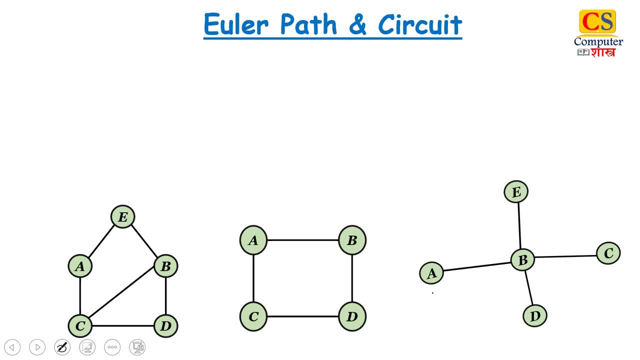 But this is a very big graph, or very complex, in which you will not explore all the paths. So for that we have two algorithms. The first is: a graph will contain an Euler path if, and only if, it contains at most two vertices of odd degree. 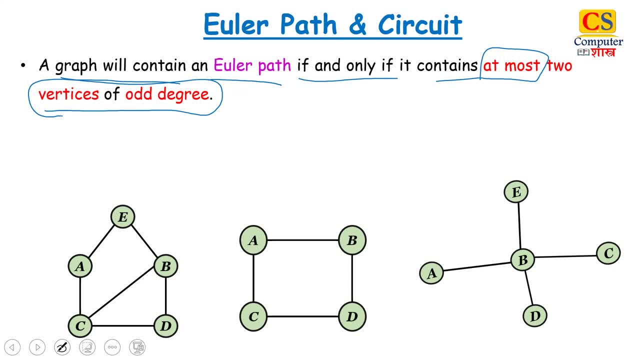 At most means maximum two vertices of odd degree. If it contains at most two vertices of odd degree, then it will be an Euler path. Now we will check in these examples whether this condition is being fulfilled or not. In the first example we will find out the degrees of all vertices. 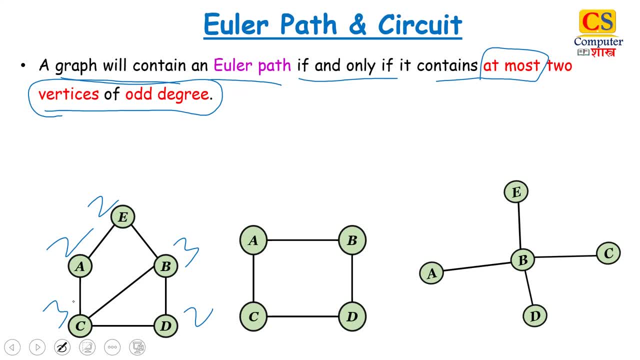 Now we have found out the degree. Now you can see that there are exactly two vertices whose degree is 3. There are not more than two Because in our theorem it is said that at most two vertices, At most two vertices of odd degree. 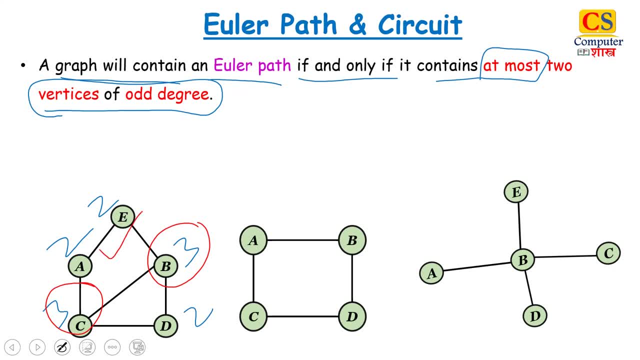 If the condition is fulfilled, then yes, an Euler path will be made in this graph. Let's check in the second graph Again. we will find out the degrees of all vertices. All vertices are 2,, 2,, 2, 2.. 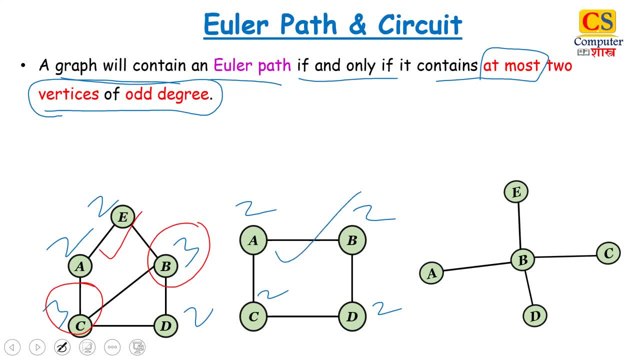 There is no odd degree. So, yes, an Euler path will be made in this too, Because it is said that at most, it is not necessary that there are two vertices of odd degree. Even if there is none, then an Euler path will be made. 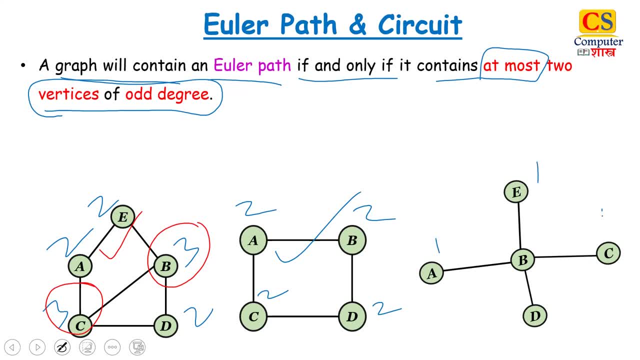 Now we will check in the last. We have found out the degrees of all vertices. Now here you can see that there are four vertices whose degree is odd. So from this we can see that there is no Euler path in this. So any graph is given. 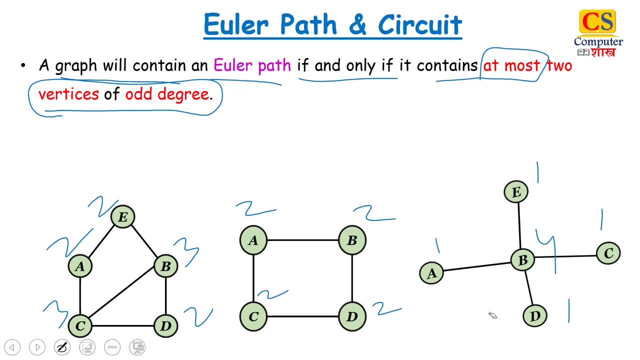 You don't have to find the Euler path. You can find out by looking at the degree whether that Euler path will be made or not. Next we will see how we will know about the Euler circuit. Now, a graph will contain an Euler circuit if, and only if, all vertices are of even degree. 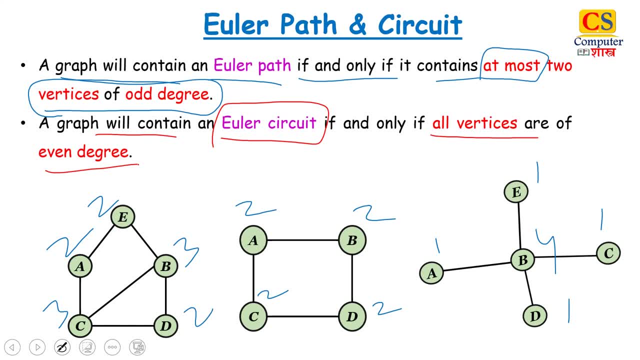 This means that there should not be any single vertex of odd degree. Now, first we will see an example. So here we have two vertices of odd degree, So we will cross it that there is no Euler circuit in this. Now, in the second graph, all vertices are of even degree. 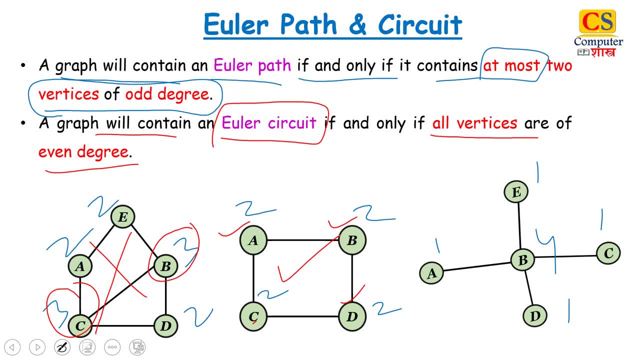 So, yes, an Euler circuit will be made in this, And if there is an odd degree in the last, then it will not be made. This is what we did at the back When we did the definition of an Euler circuit and did the examples. 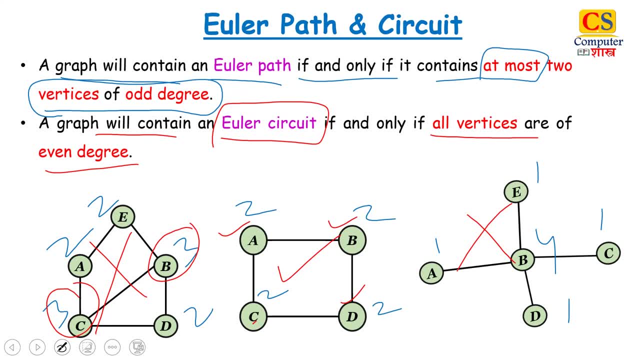 that only in the center there will be an Euler circuit and not in the rest. We are proving the same with theorem Now. we will do some practice problems in the future. then you will know how useful this theorem is. Next we have a term called Euler graph. 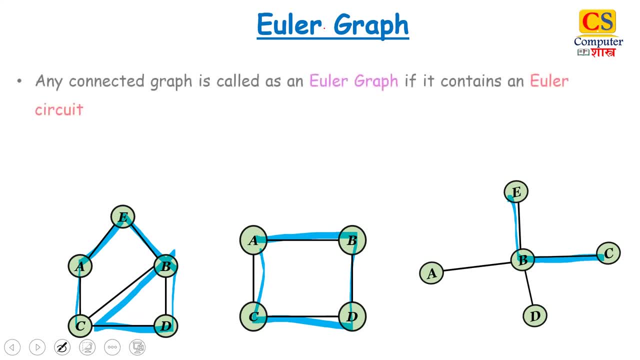 Euler path is made and circuit is made. Now what is Euler graph? Any connected graph is called as an Euler graph if it contains an Euler circuit. If there is an Euler circuit in any graph, then we will call it as an Euler graph. So will we call the first graph as an Euler graph? No, 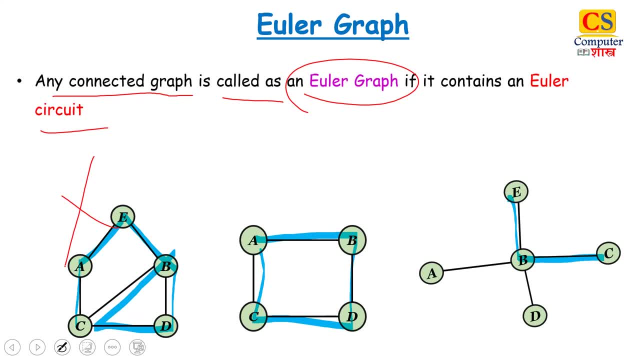 Because there is no Euler circuit in it. It is just an Euler path. Second graph: Yes, Because there is an Euler circuit in it. Third: No. So among these three graphs, only the second graph is an Euler graph, Clear. Next we will see some practice problems. 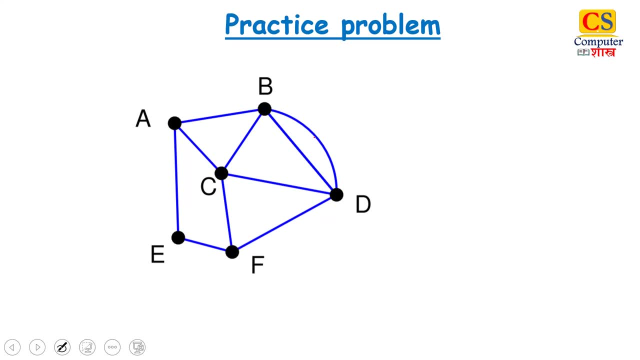 This is my first problem In this. we have to find out whether there is an Euler path, an Euler graph or an Euler circuit, What is an Euler circuit and what is not? So, again, we will find out the degrees of all. These are the degrees. 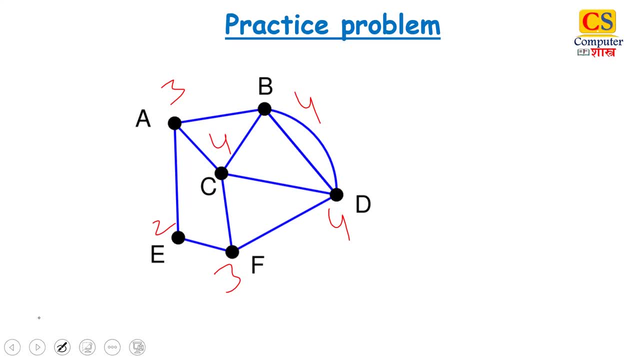 Now we will check what is the odd degree. Now there are only two odd degrees in this graph. Whenever there are at most two odd degrees, then we know that it is an Euler path. Now in this graph there will not be an Euler circuit. 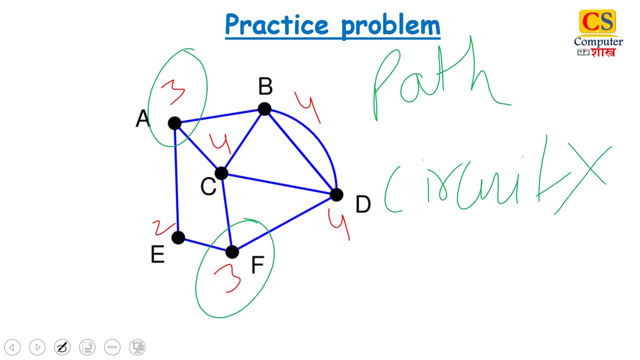 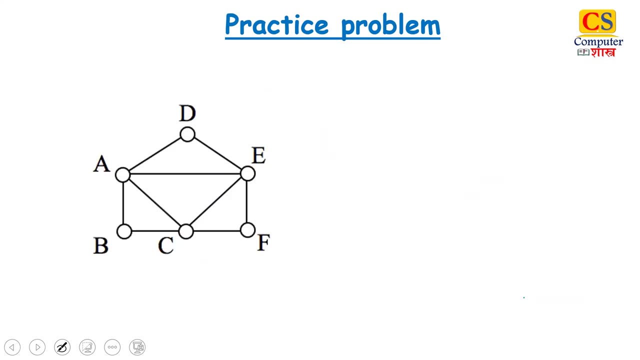 There will be only an Euler path. Now, if there is no Euler circuit, then we will not call this graph an Euler graph. We will know all the things in this graph. Let's check one more problem. This is my next problem. Now this graph is even. 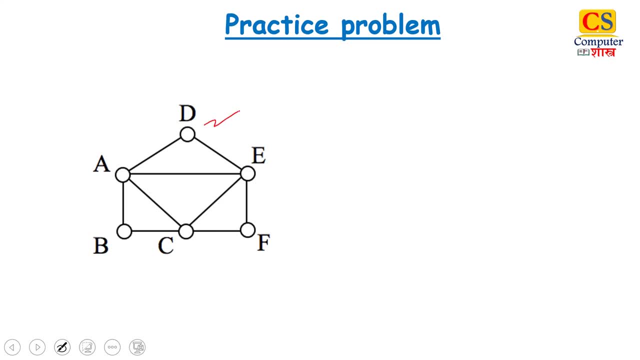 We have to check what will happen Again. we will find out the degrees. Now, in this, all the degrees are even. So now what will we say? Will this be our Euler path? Look, A circuit will be formed, because the circuit is saying that all the degrees should be even.